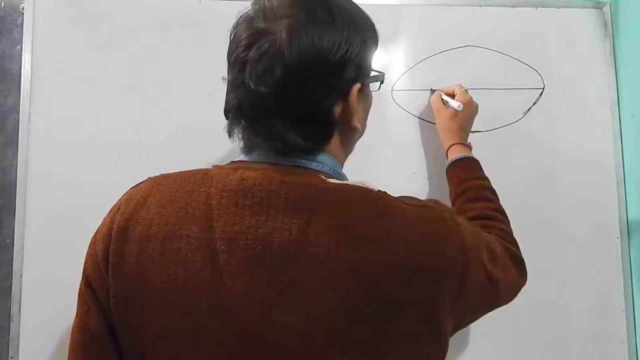 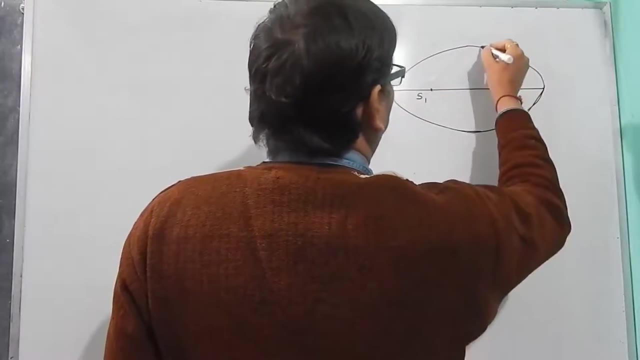 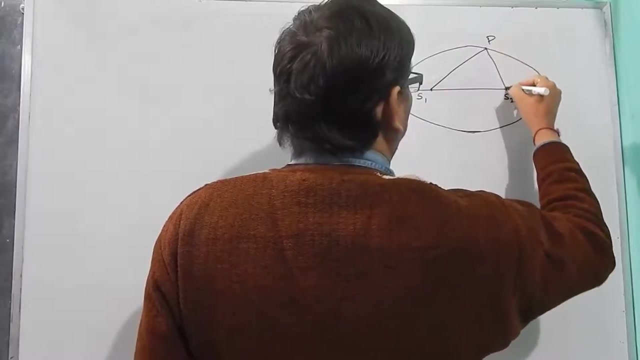 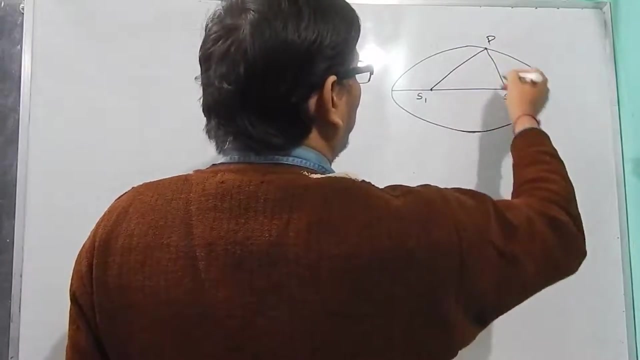 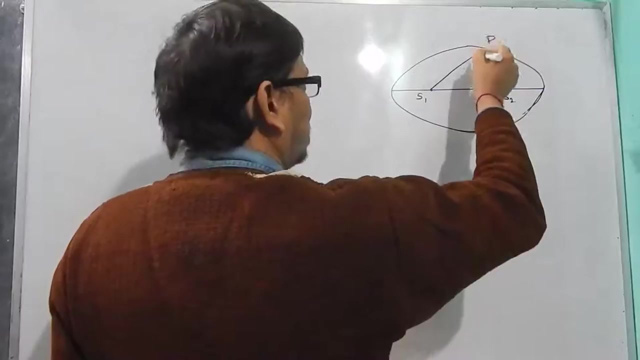 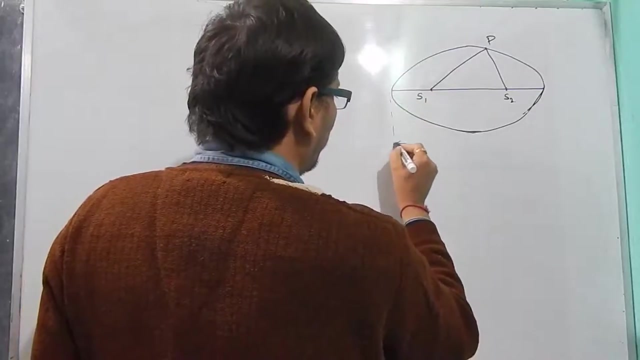 So the property is like this: If suppose this is one focus, S1, and this is another focus, S2.. So you must be knowing that from the conic section, that if any point is taken on the ellipse, So this distance P S1 plus P S2.. So sum of these two distance, P may be anywhere but the sum of the point from one focus plus the distance to the other focus. So these two distance is equal to the distance of major axis. 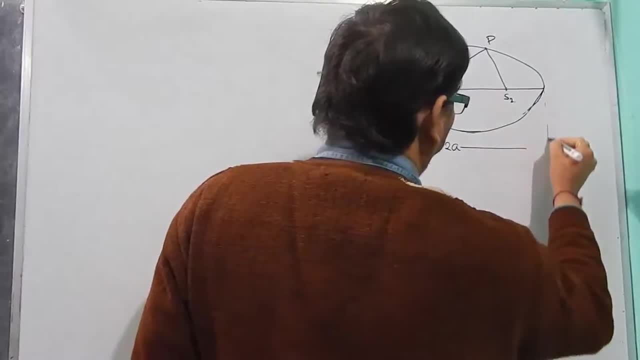 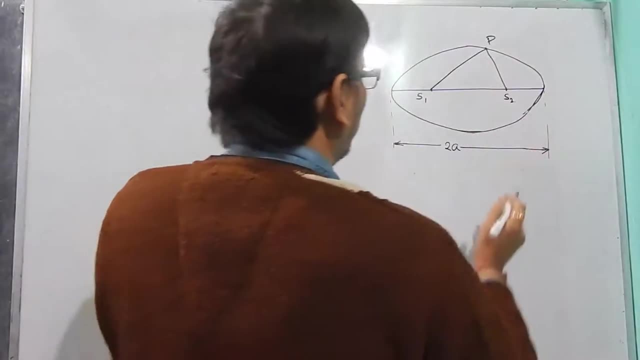 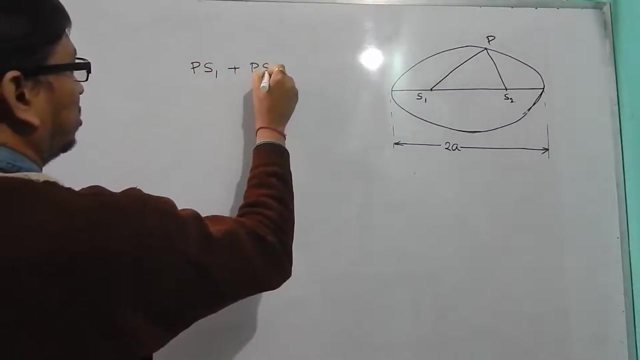 2 is that of the major axis, means 2A. So P S1 plus P S2 always will be equal to 2A. So this is the property of ellipse. So we use this property to find the locus of point P when we use complex number. 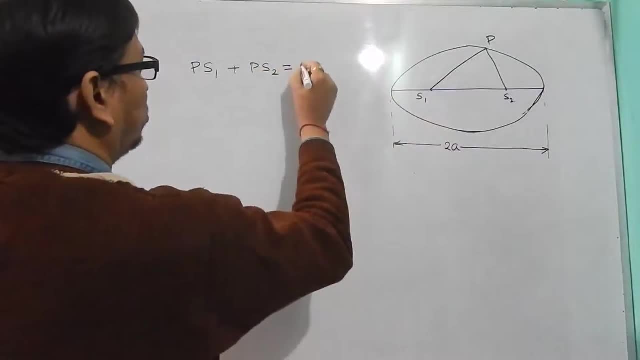 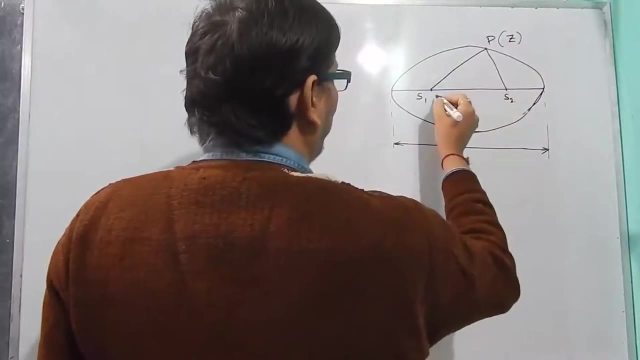 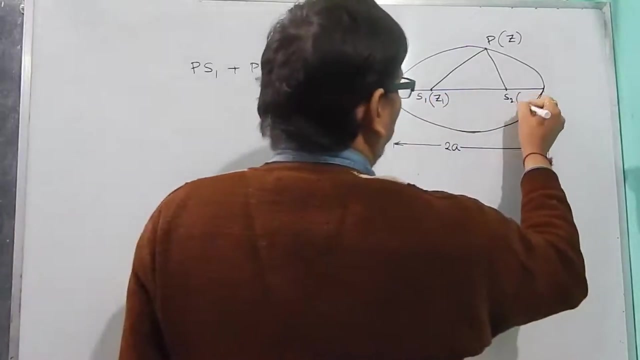 So P S1 plus P S2 will be equal to 2A. So if we take this is a complex number, Z, The locus of which is to be find out, And suppose S1 is another point that is the focus, Z1, and S2 is another point, which is Z2.. 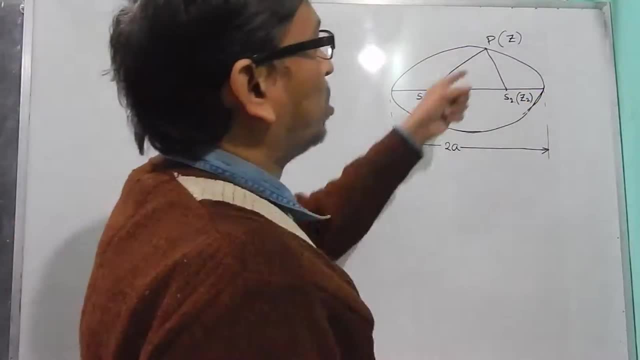 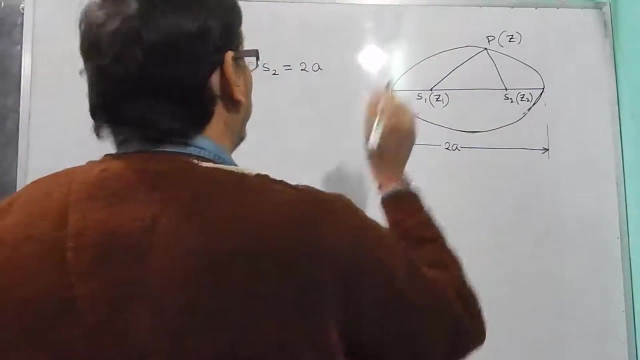 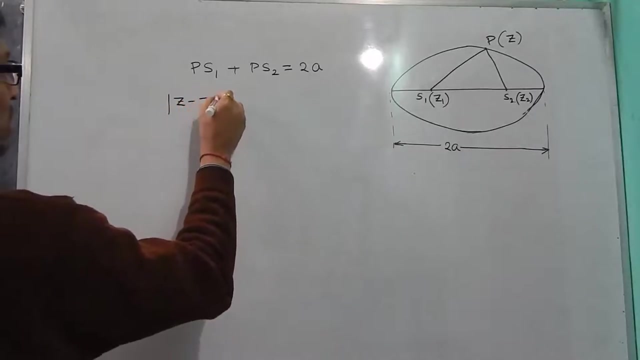 So we are interested to find out The locus of Z, where Z1 and Z2, these two foci are already known, So these two should be known. So then you can find the locus of this. So that means P S1, the distance, P S1, that is Z minus Z1 plus P S2.. 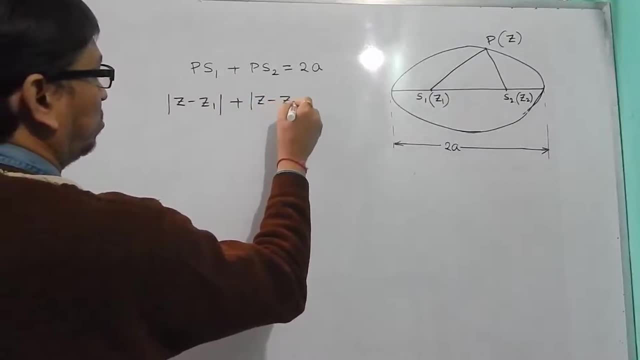 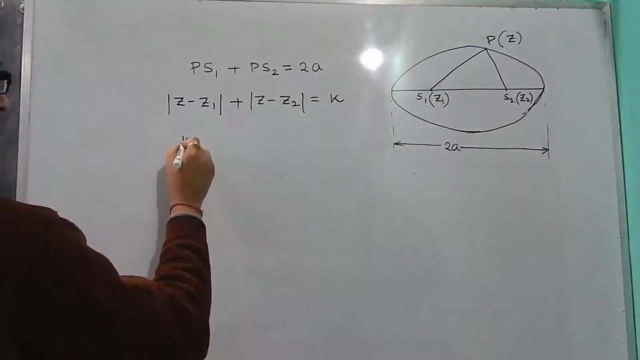 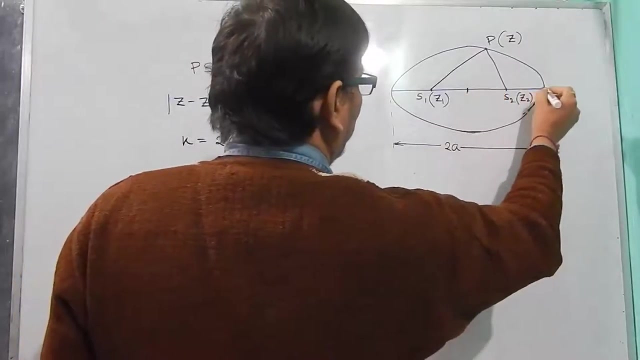 So that is Z minus Z2.. So this should be equal to 2K. So we write it a constant. So where this constant actually K Is equal to, Is equal to twice A. A means its semi major axis, means this distance. 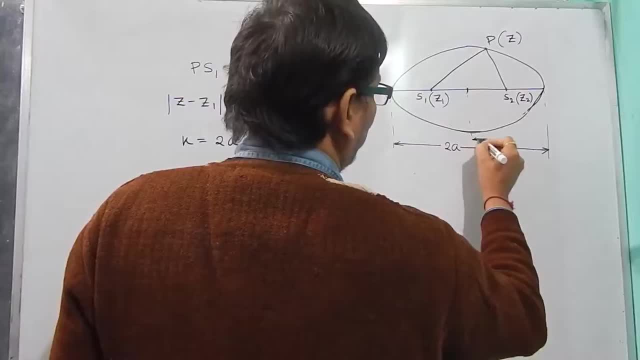 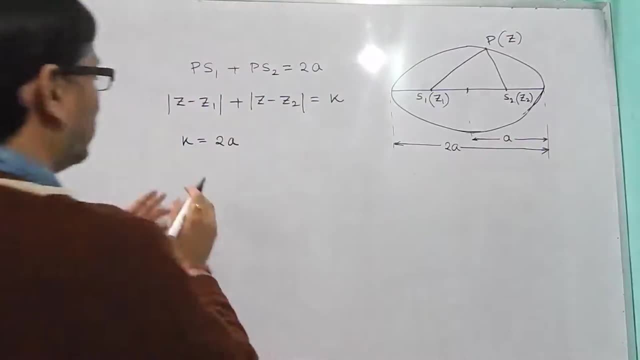 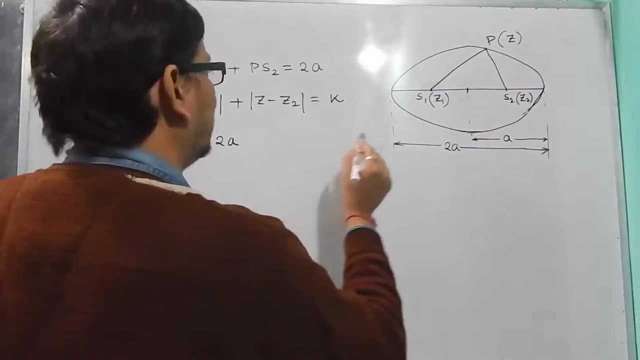 So from here to the end this distance is called semi major axis, So this distance is A And the total major axis is 2A, So K is equal to 2A. So what thing is to be maintained here that the distance between two foci? 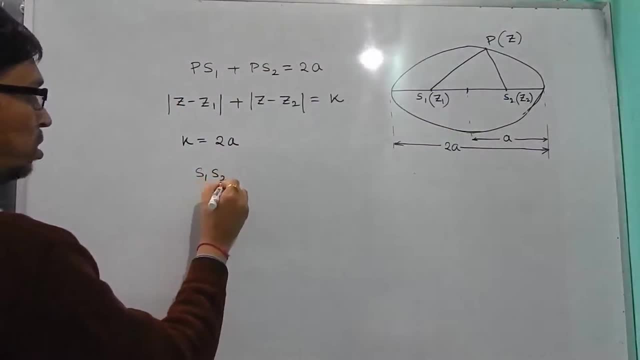 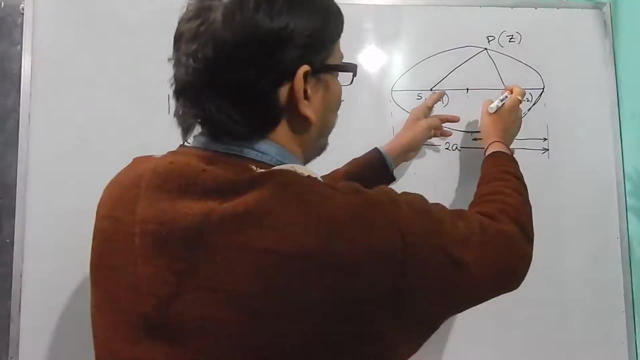 That means S1- S2.. S1- S2. Must be always less than 2A, Because this is the distance between two foci And this distance must be less than its major axis. So S1- S2 must be less than 2A. 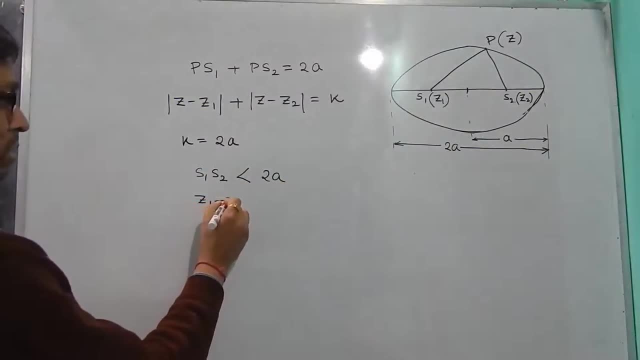 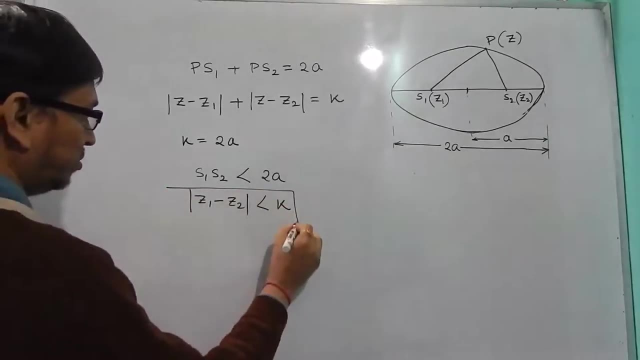 So S1- S2 is Z1 minus Z2.. And the modulus of this this is the distance, So this must be less than K, So this is to be maintained. So when you find this is the equation of an ellipse, Z minus Z1.. 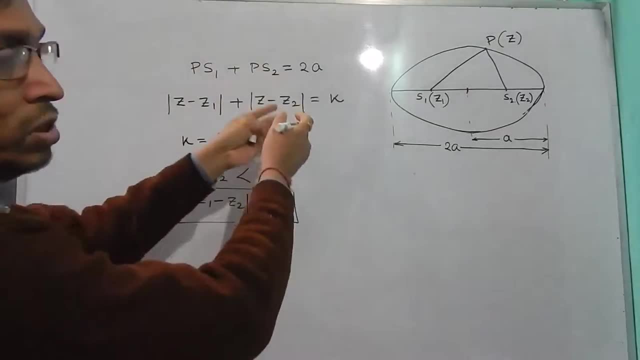 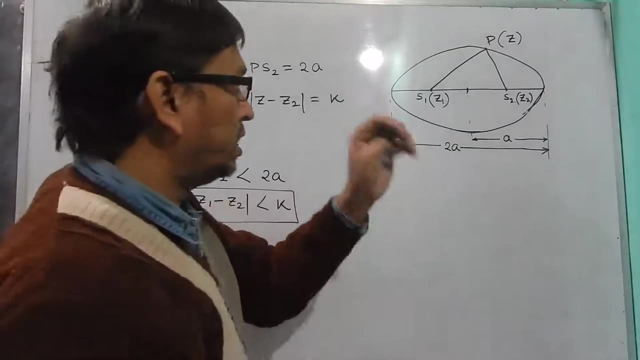 Plus Z minus Z2.. Modulus of this two is equal to K. Then you have to notice at first Whether Z1 minus Z2 is less than K or not. If it is less than K, That means it is ellipse. Now say in case of hyperbola: 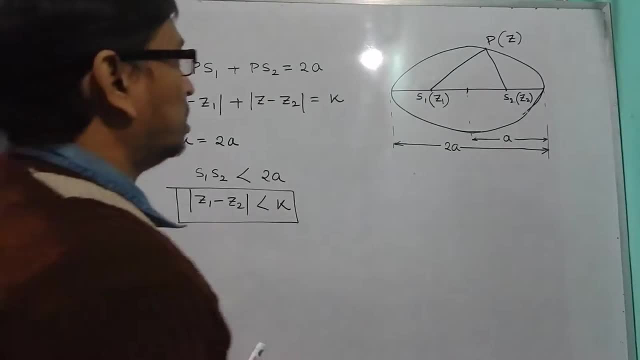 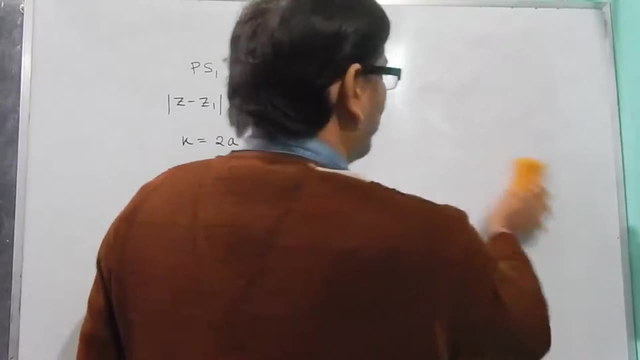 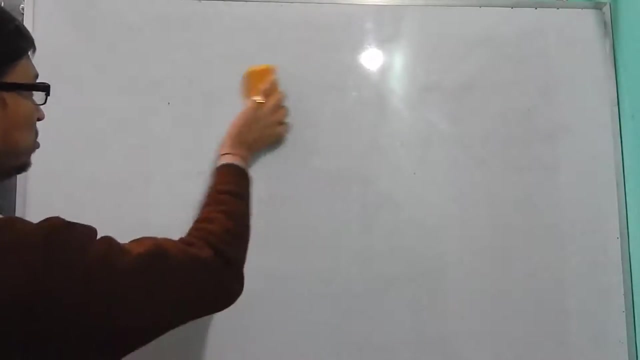 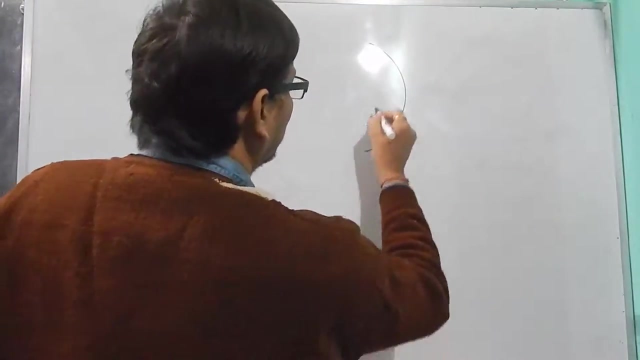 So in case of hyperbola, The thing like The thing changes And it takes the form like this. So you have to make your own concept at first. So suppose this is This one is hyperbola, So you consider this is as hyperbola. 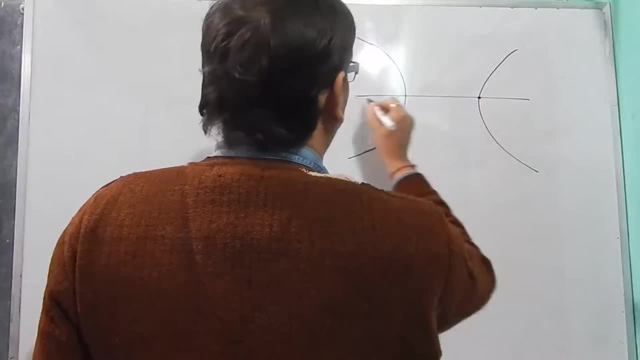 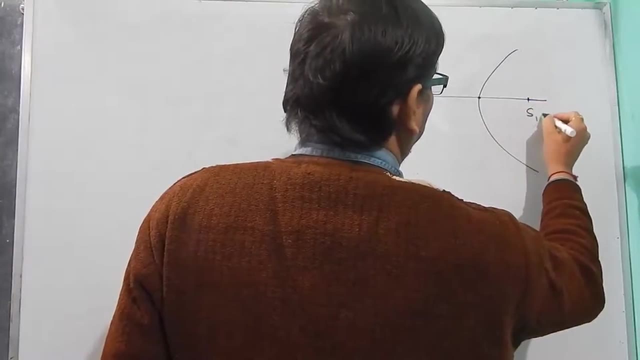 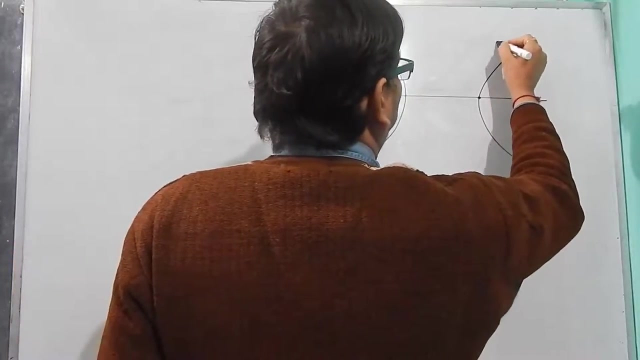 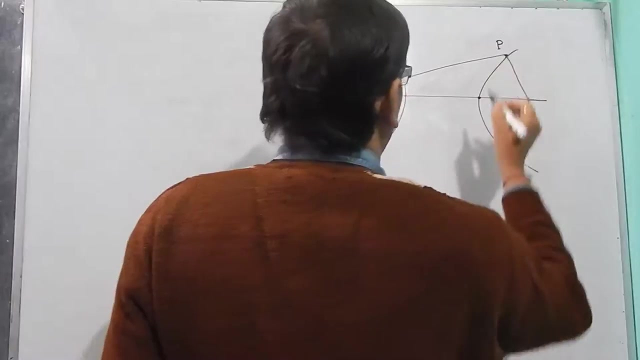 Because this is hand drawing. So here also You will find: here is one focus, Here is another focus. So suppose this focus is S1. And this focus is S2. And here it is a point, say P. So in hyperbola what is maintained? 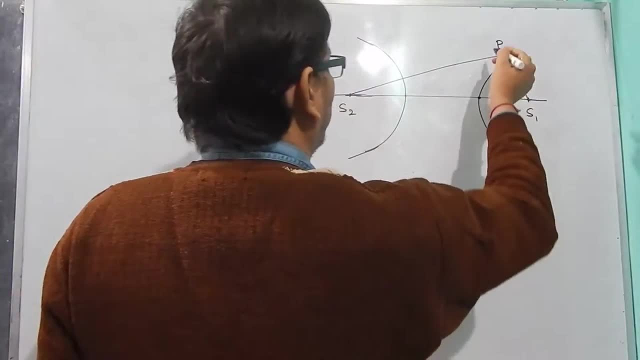 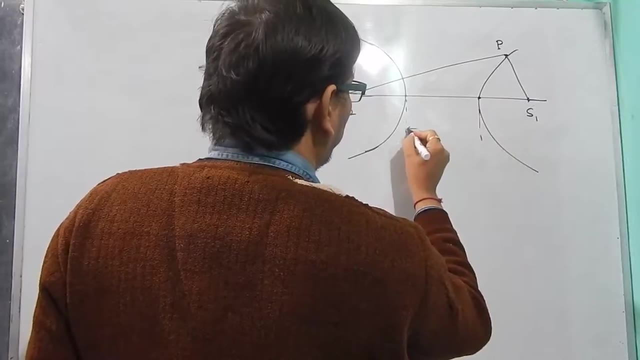 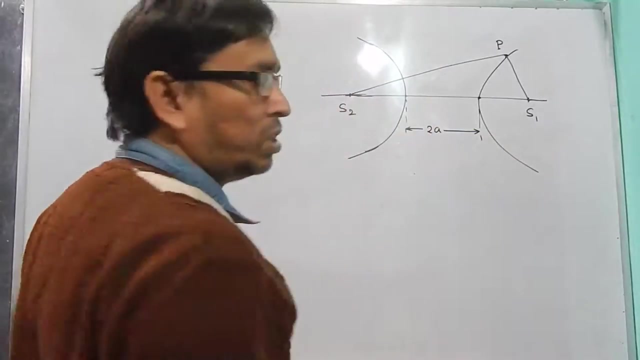 So P S2 minus P S1.. So the distance: P S2 minus P S1.. This will be equal to the distance of its major axis. Here its major axis is this much, So this is its two In hyperbola, if you know the conic section. 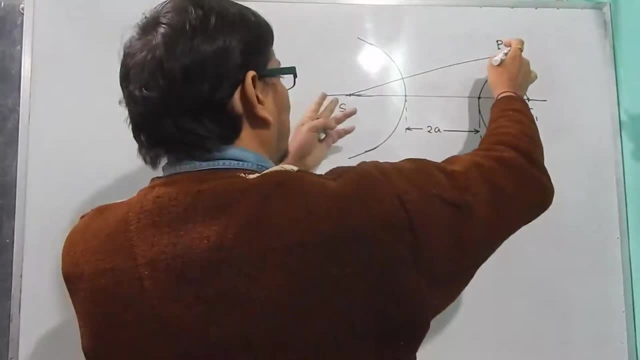 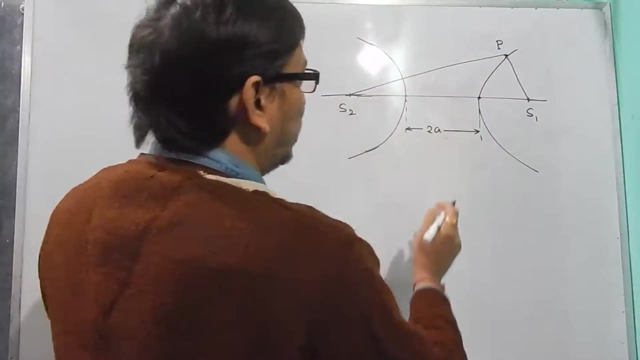 Then you must be knowing that P S2.. That is the larger length From the point to the one focus, Minus the smaller length, That will be always equal to 2.. So we can write P S2 minus P S1.. 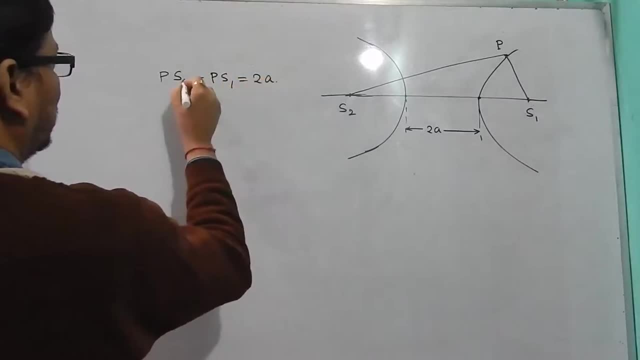 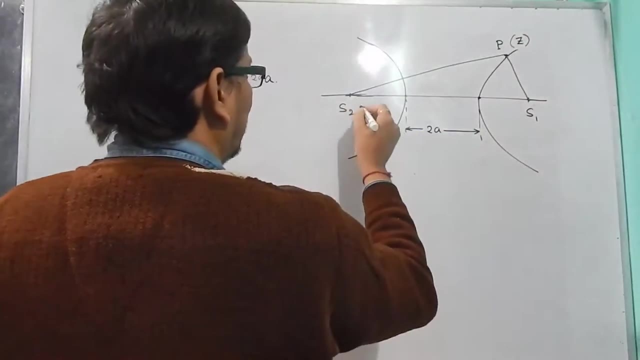 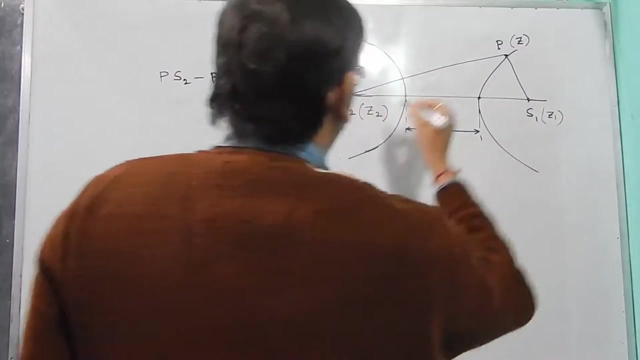 Is equal to 2A, So P, S2.. Suppose this point is Z, So the locus of which is to be determined. And this point, suppose Z2.. And this point, suppose this, is Z1. So the thing will be like this: